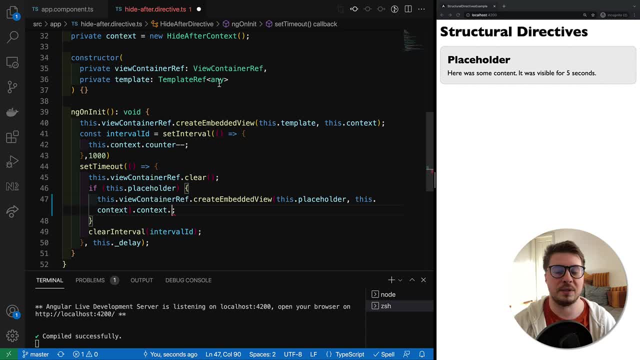 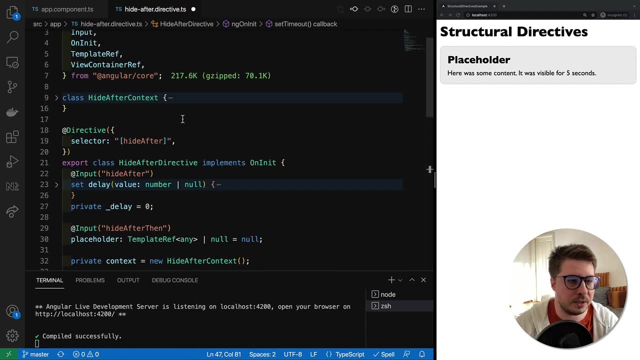 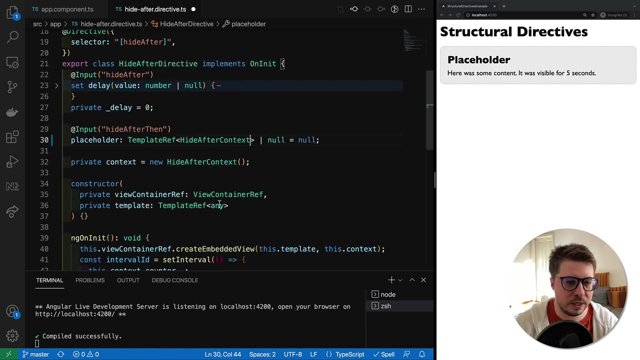 no suggestions, So you can go to the context. We don't have any suggestions because the type is any. We don't know what is inside this property, So it is quite easy to fix. We just have to copy the class name and replace our any with the hide after context. 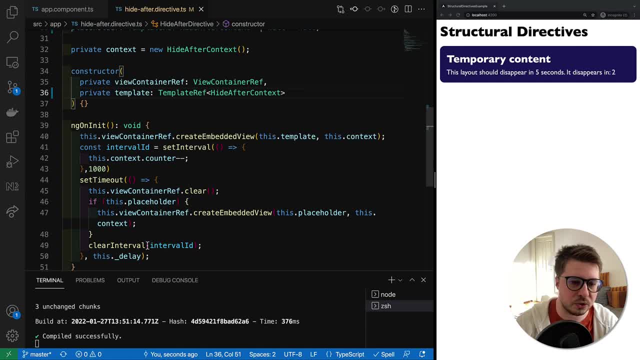 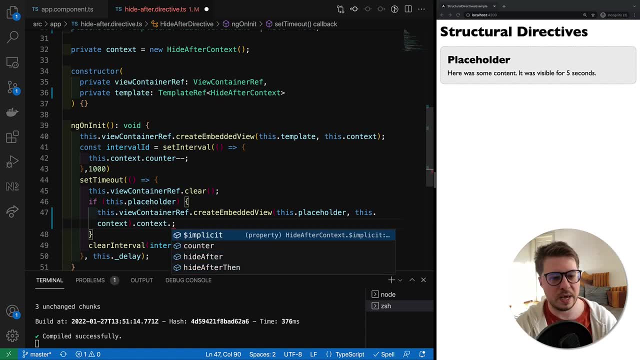 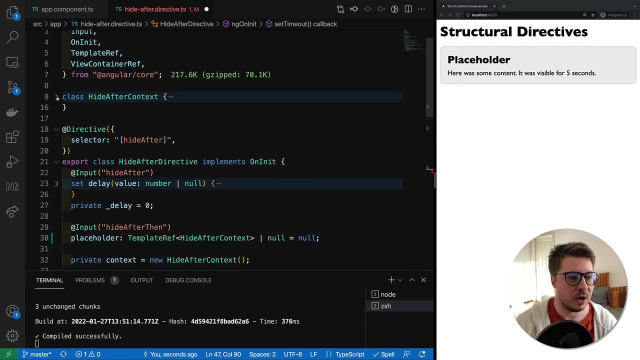 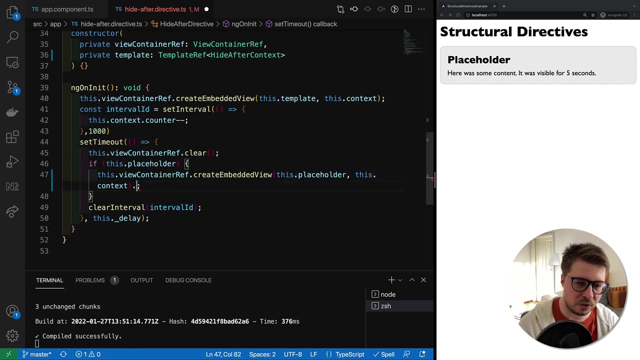 And now, if we save and if we try to access the context right now, We can see that We have suggestion regarding the properties which are available for our context. We can see all of them right here. So this way you can achieve better typings in your structural directive in your context. 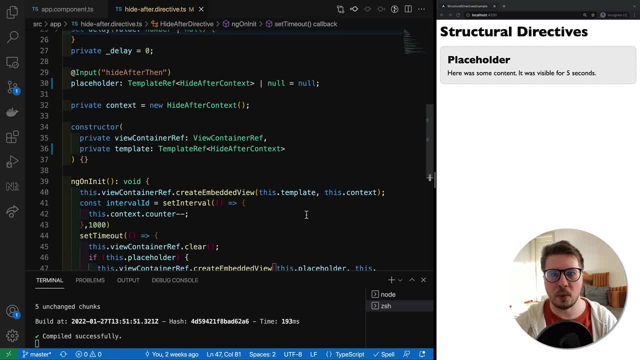 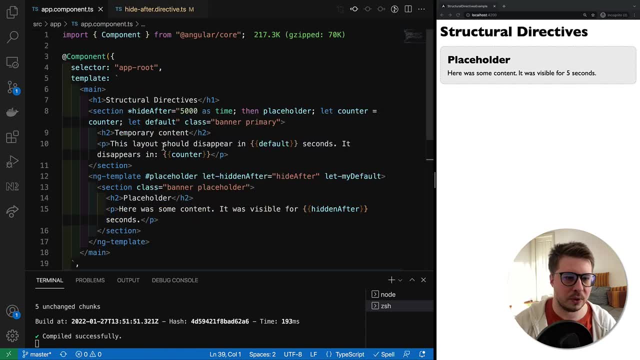 So this is the really easy part and let's move forward and I'm going to show you one interesting use case. So Let's go to our template and you can see that I'm using the counter here. Yeah, I introduced variable inside my template counter and assign the counter which comes. 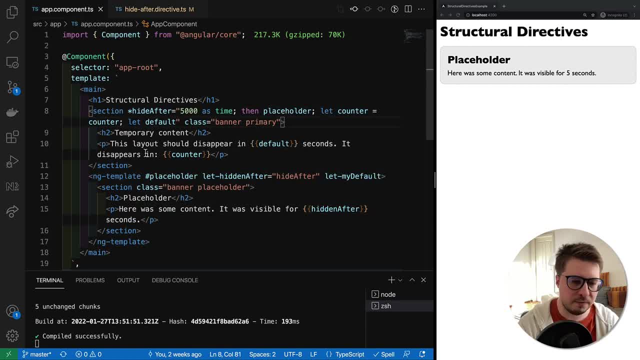 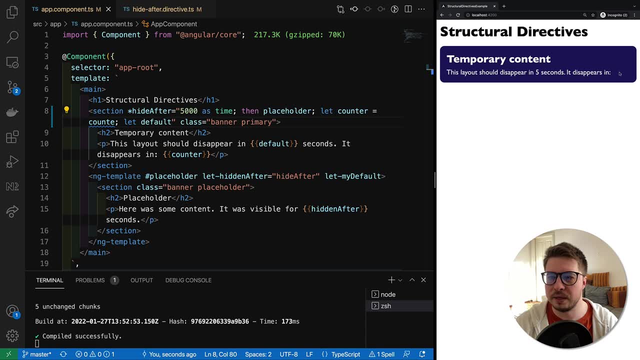 from the context, Right, But what if I did some typo here? If I save it, you can see that our directive works not as we expect. We don't have a counter here And Angular compiler doesn't Take. Tell me that I made a typo. 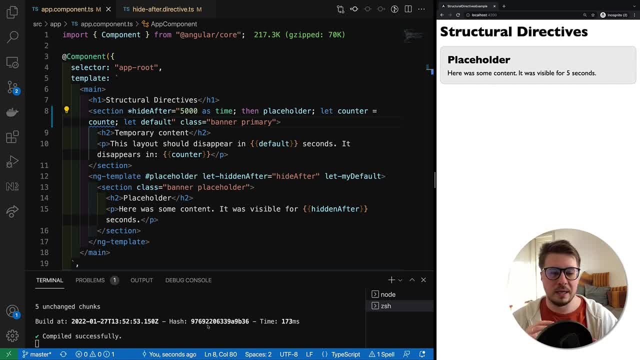 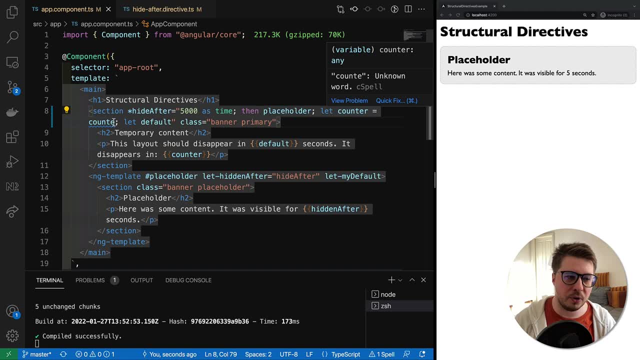 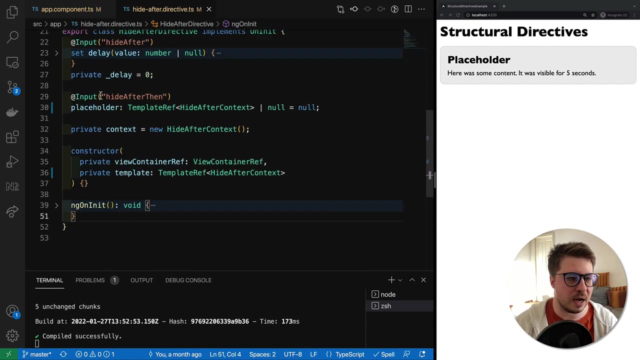 So it would be great to have some guard which could catch this case and indicate that we had a typo here or we're trying to access context variable which doesn't exist, And in order to achieve this we have to introduce a new static method in our directive class. 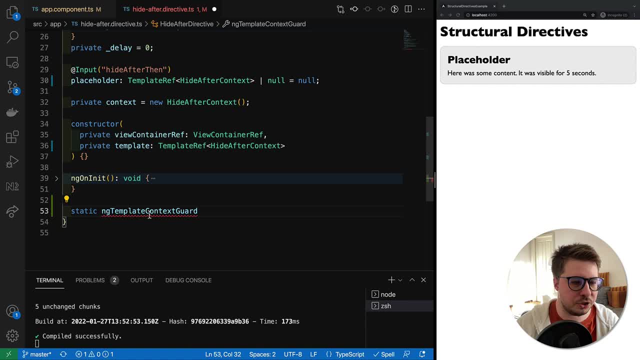 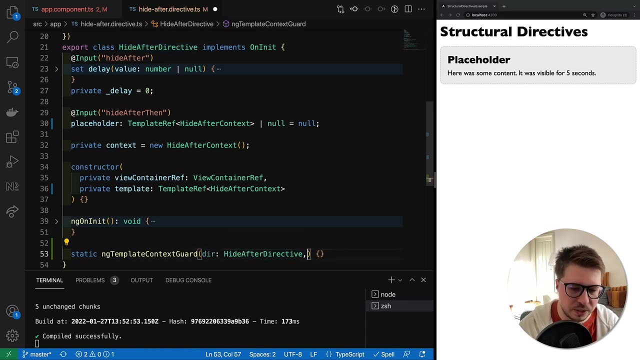 And namely this method called ngTemplateContextGuard. And this method takes two arguments. The first one is a directive itself- It's going to be our hide after directive, So I paste it here. And the second argument is the context, which is going to be unknown. 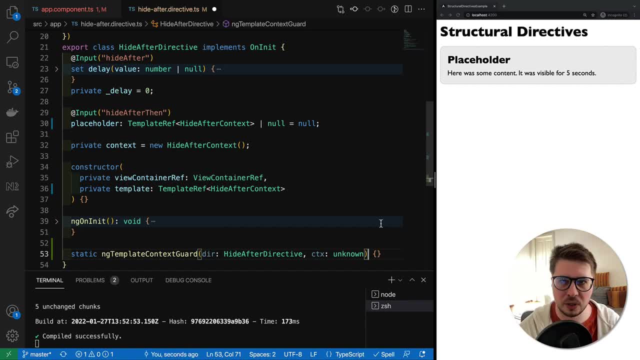 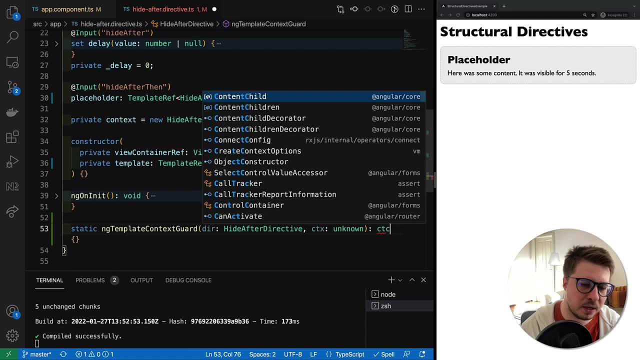 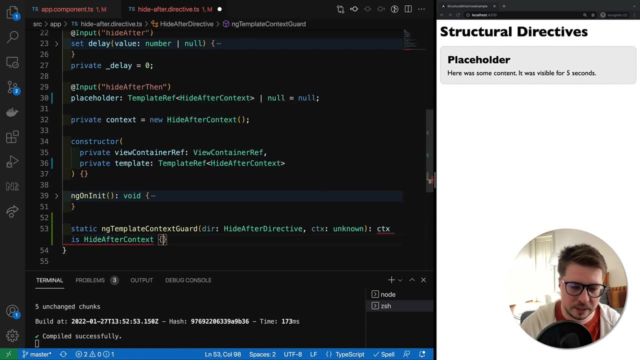 Then we have to do the next trick. I will write it and then I will explain. It will be easier to understand. So we should say in return type: that context is our hide after context And then we say just return: true, What's going on here? 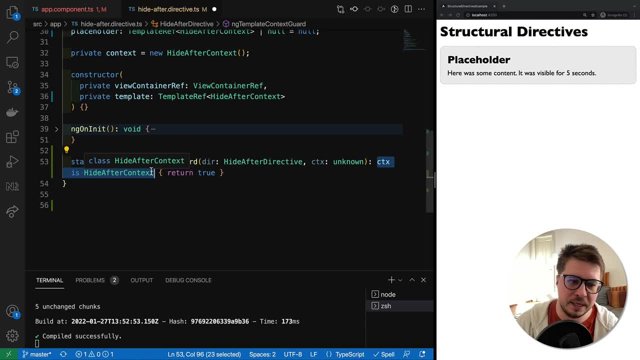 So it is so-called type predicate in TypeScript, And if you know what is that, you can use time codes In the video description and skip this section. for those who sees first time this magic, I will try to quickly explain how it works. 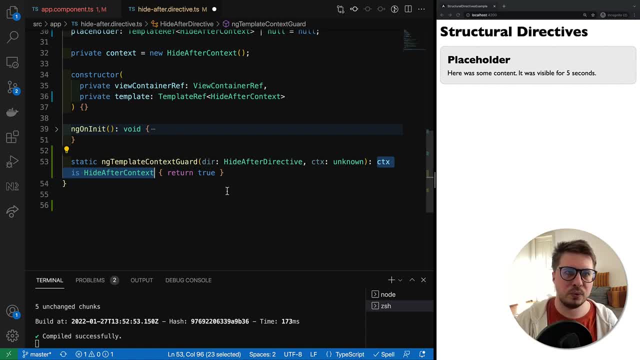 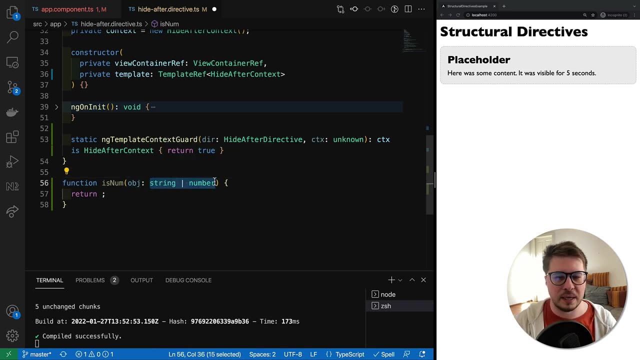 So we use the type predicate if we want to check if something belongs to some certain type, As example. as example, we have some function called isNum whatever which takes the object which has a union type. So it might be either string. 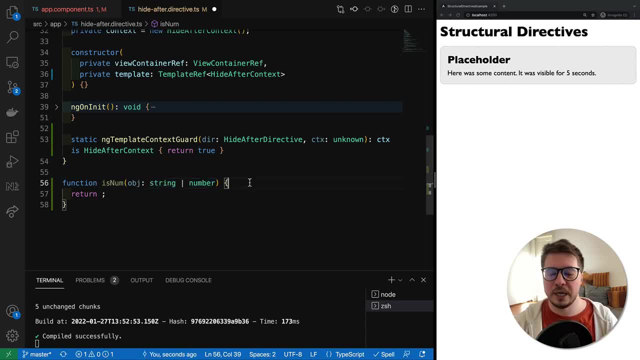 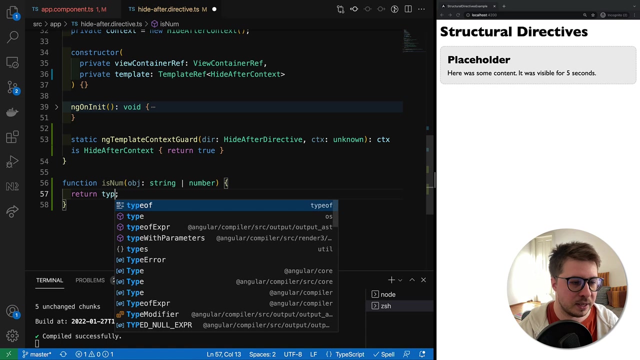 Or it might be a number, And imagine that in runtime we have to check somehow which type this object is. So first of all what we have to do is to do some simple check and return true or false. So in our case we have to check is if type of object is number. 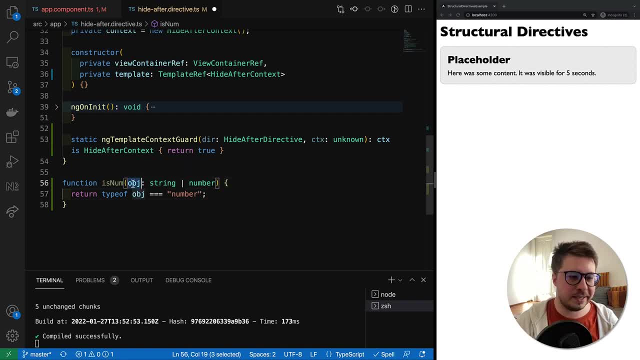 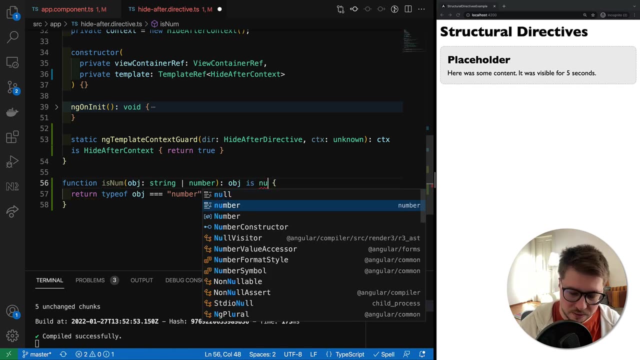 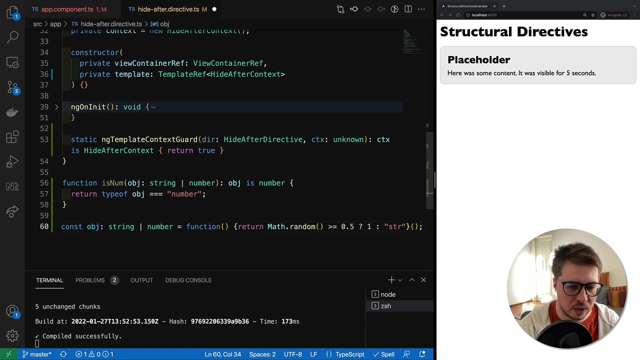 And then we should tell TypeScript that object is a number. So that's why we as a return type define, type predicate and say that the object, so basically this object- is number. So now we could have something like constant object, which is either string or a number. 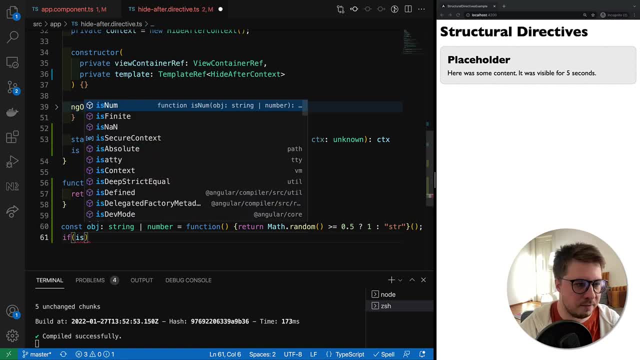 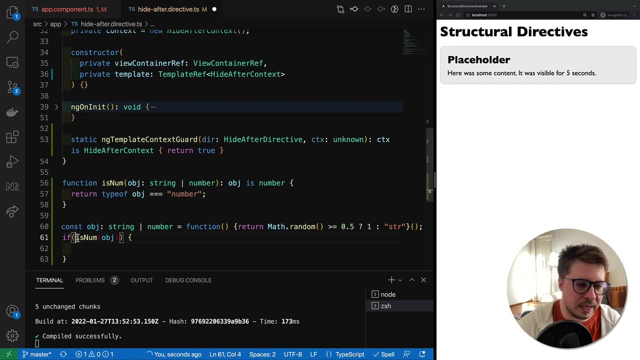 And then we might have some check Like: if is number. And then we might have some check Like if is object a number, And in this case TypeScript knows that if this function returns a true, it means that the object is a number. 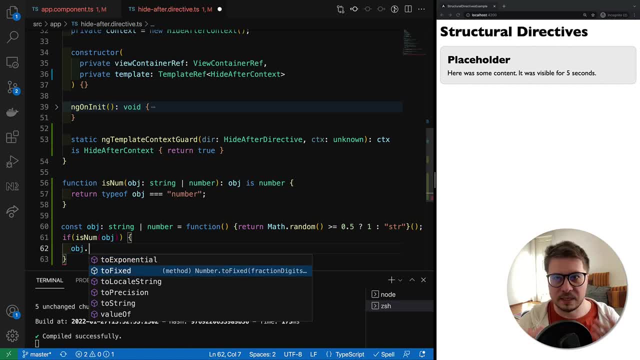 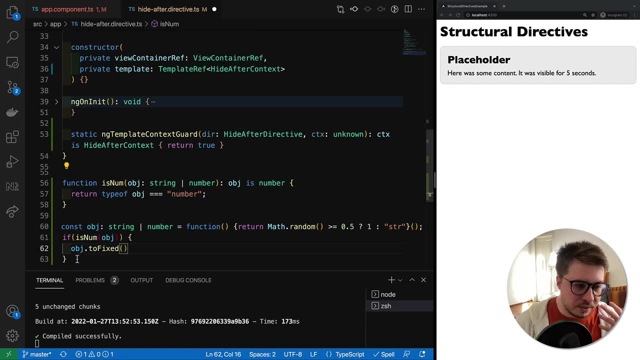 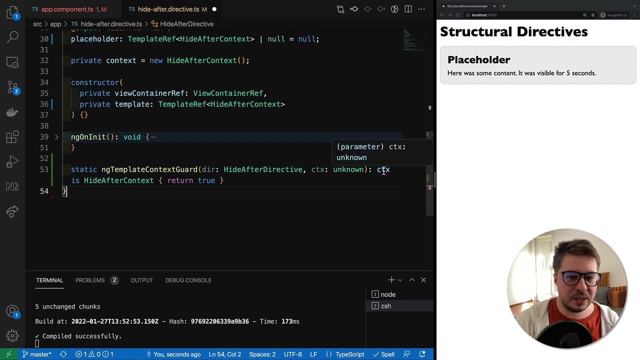 So we can safely call some method which belongs only to number, So like that. And this is how it works, And this is exactly what we do with our ngTemplate context guard. So, basically, we return true, which means that our context is going to be hide after. 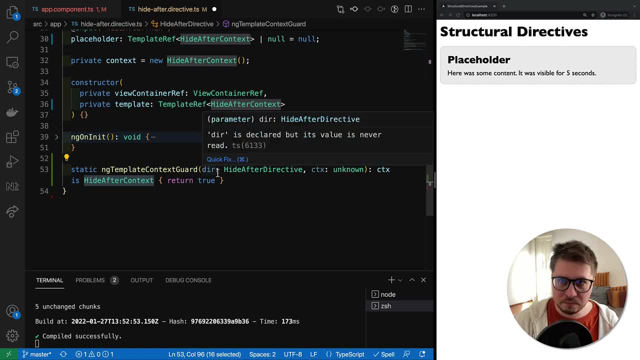 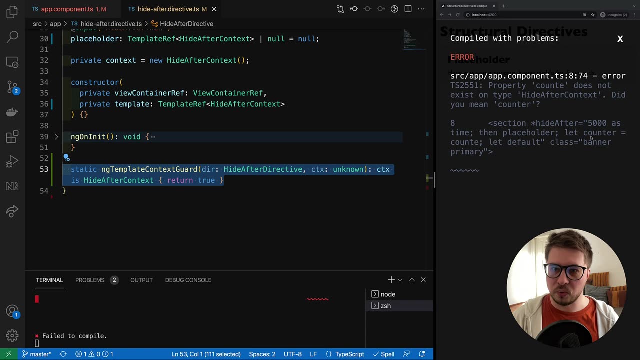 context. You can do more complicated check actually, if you need, But in our case we always, we always have hide after context. So this construction is absolutely fine in our case. we can save it And now we can see already the error which throws Angular compiler to us, because it's 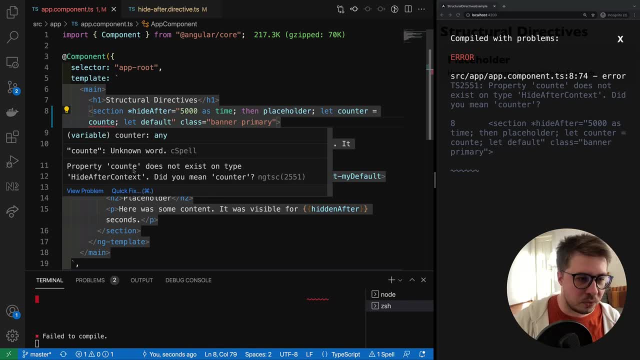 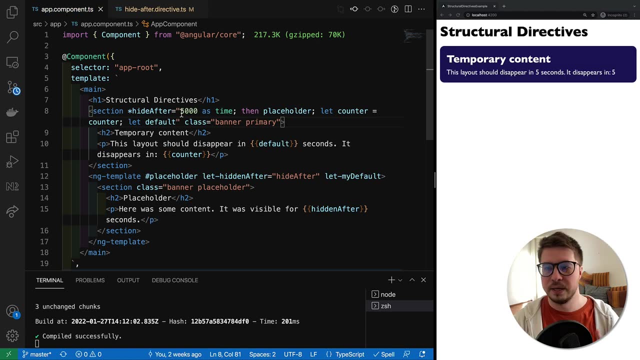 says that, all right, the property counter does not exist. did you mean counter? of course I meant counter, and now, if I save it, we see that everything works fine again and directive works properly. it is already super cool and there are a lot of use cases where you can utilize. 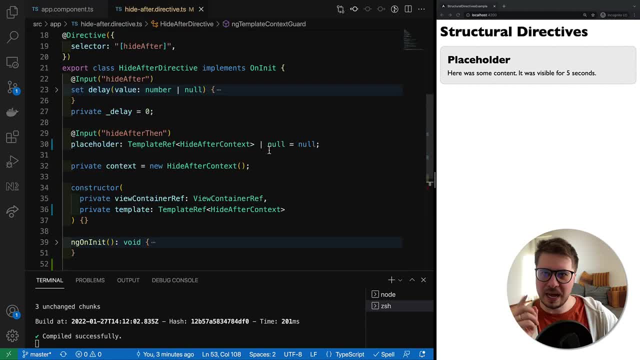 that type guard for your context. but I would like to show you one more cool thing which you will be using, probably not so often. this is really quite rare cases when you would need it, but still, I will try to explain it to cover this topic about directives completely. 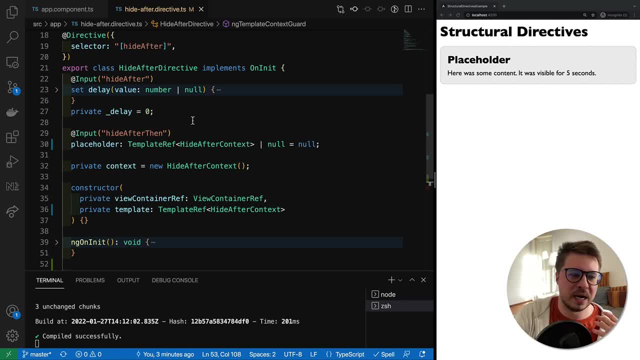 and I'm talking about narrowing type for our inputs in structural directives. so I was thinking a lot what kind of feature I could introduce for this directive in order to demonstrate you this use case. I gave up. I could not come up with some meaningful idea, so I decided. 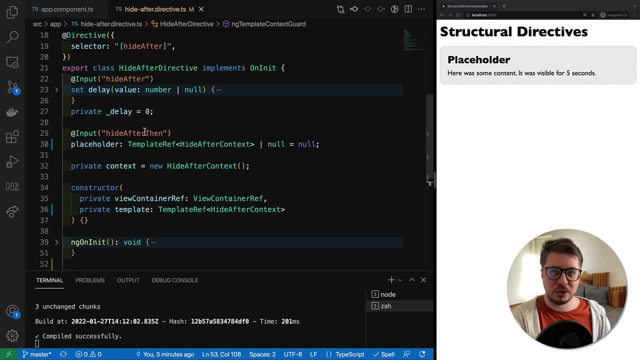 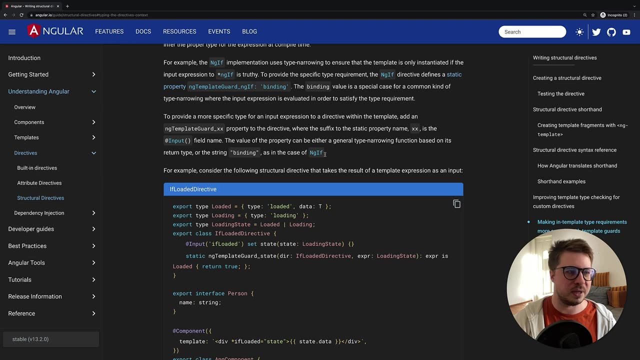 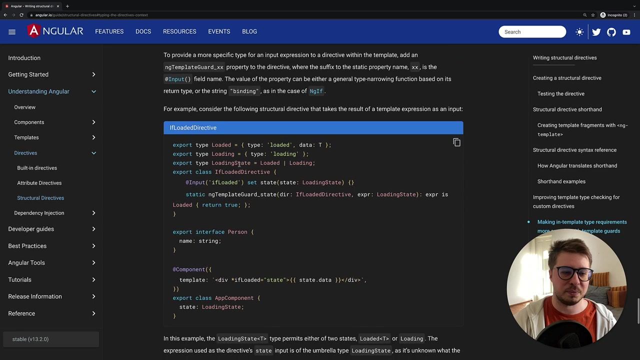 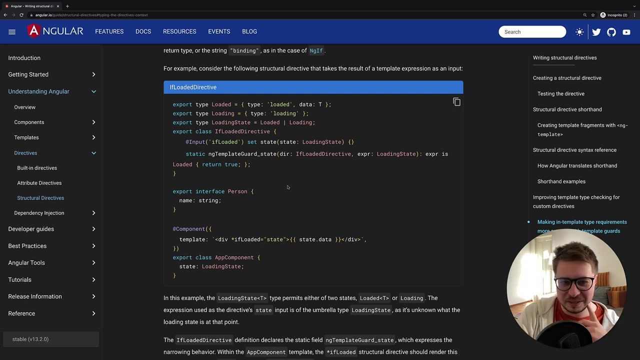 to take the use case from official documentation, because those that use case was perfect fit for this type, narrowing, however, the problem with this example, which you can find on official angular docs, and I will drop the link in the video description to this part. the problem is that this section probably is not finished yet, I suppose, because 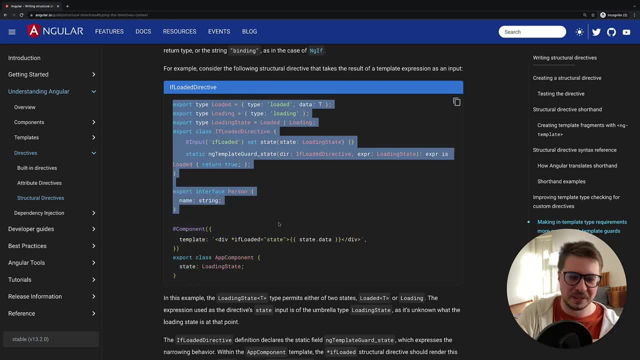 this code is. I would say this is a pseudo code. it's not something you can copy and just paste and it will work. so you have to adjust it a little bit and we'll do it right now, and once we make it work it will be pretty much clear what does this type narrowing for inputs, and in which case you. 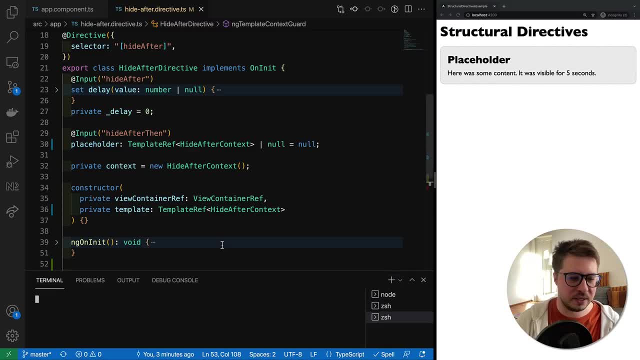 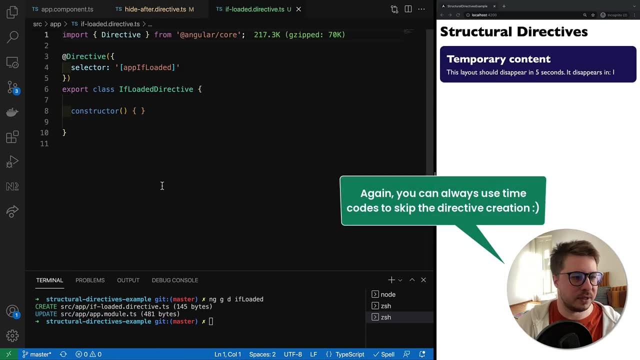 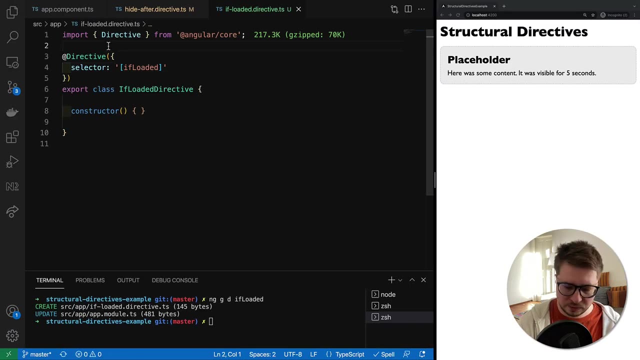 could use it. so I go back and I will generate a new directive. so call it if loaded. here we have this directive and now let's- um, maybe copy it piece by piece. so first of all, let's copy and paste our types. and here is the first problem: that we define data as a generic. but in order to use this generic, 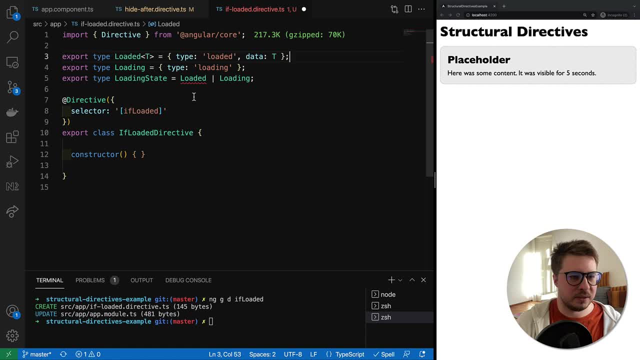 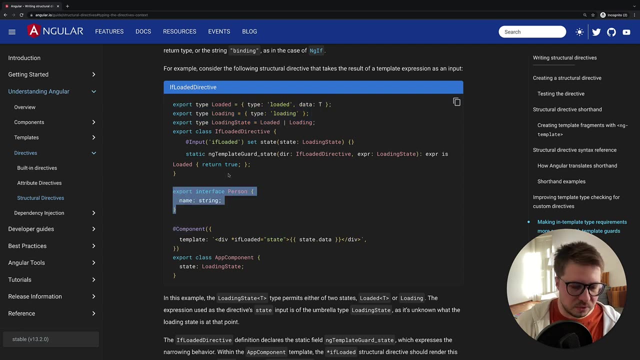 we have to declare it right here. so this is the first problem. our loading stage should be also generic, and here as well. all right, we are done with that. so let's go back to our project and let's go to our taskbar and we're done with types. then we have to import. then we have to import also. 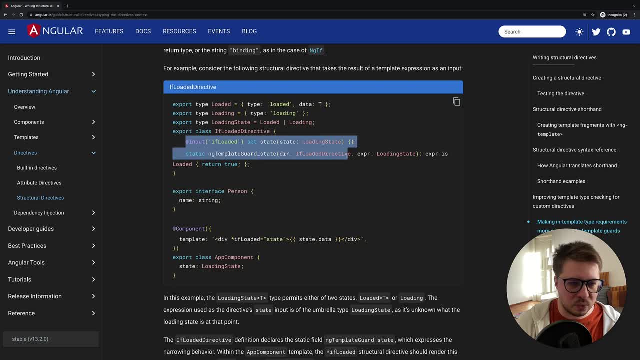 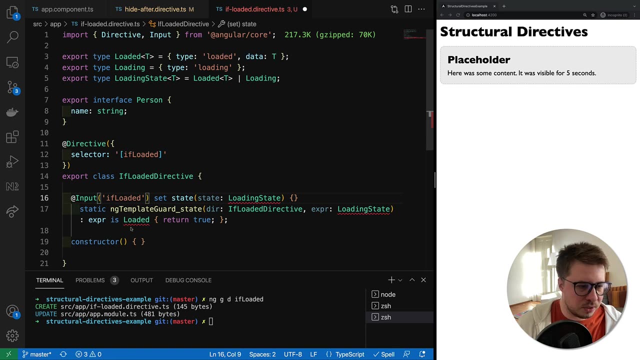 interface person. let's drop it also somewhere here. and we also need to copy the content of the if loaded directive class and this component we don't need actually, so paste it here. we have to our loading state, also generic, so let's add it here and we have to declare this: 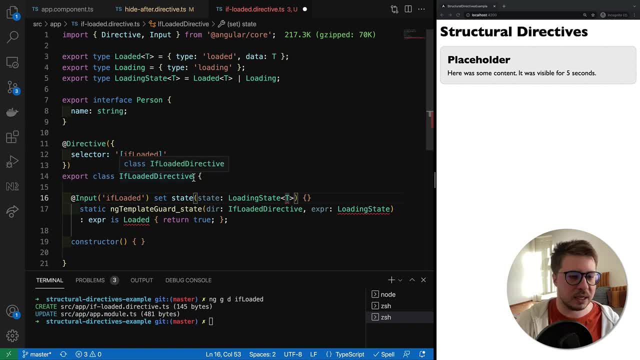 generic for the class, and for the class we can define it right after the class name, like that. and here we also have to use generics. so I will replace it here. and we have to also declare it for static method. right there, cool, we have figured out with types, and now we have to actually bring some logic to this. 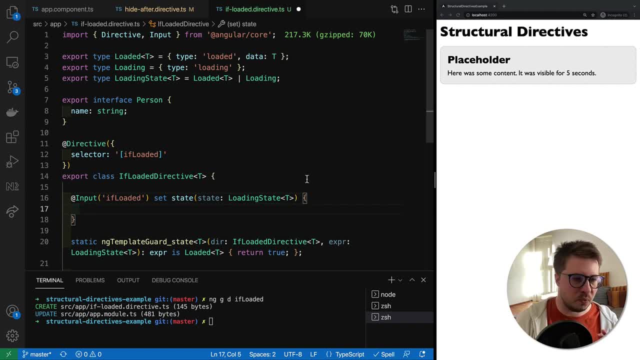 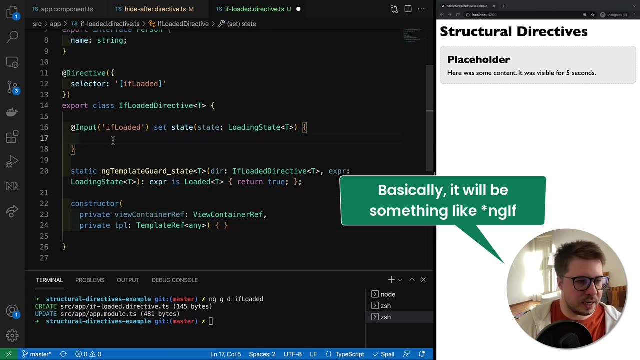 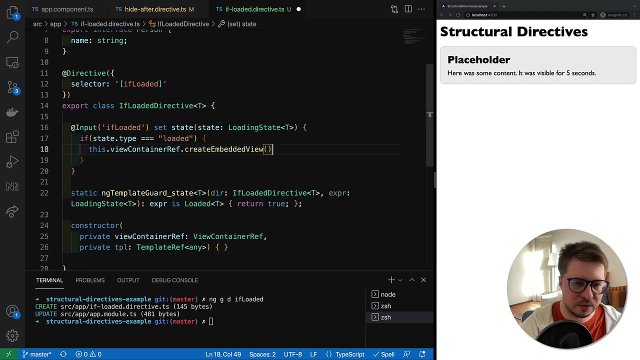 directive and logic will be very simple: once we have loading type, we don't render template. once we load it, we show some template. so let's inject view, container, ref and template and inside our input we will do very simple check that if state type equal to loaded, we going to create embedded view and render this template. 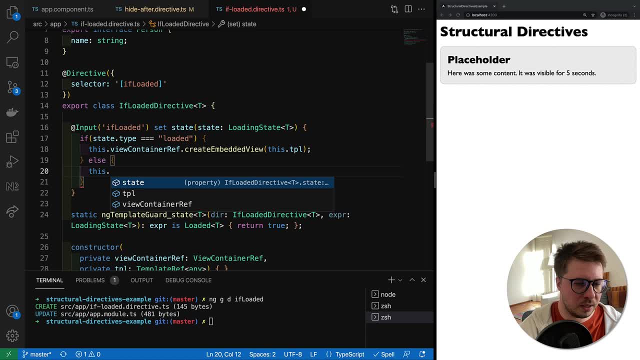 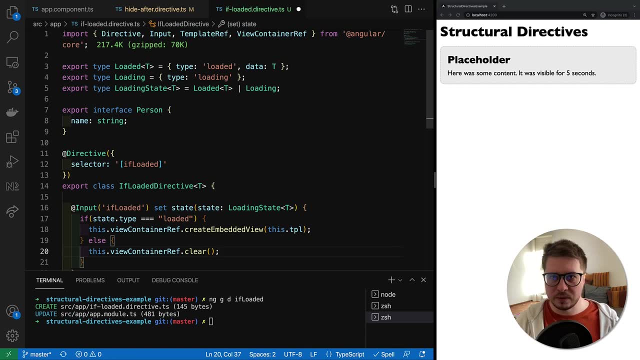 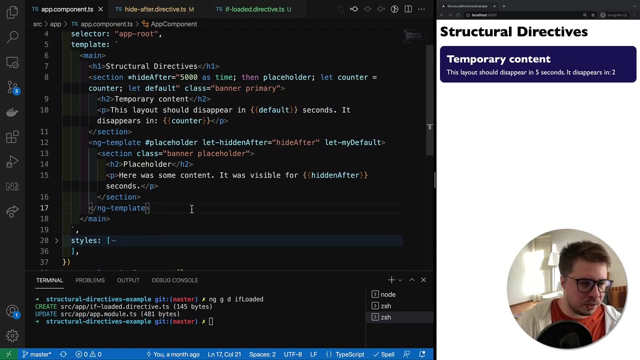 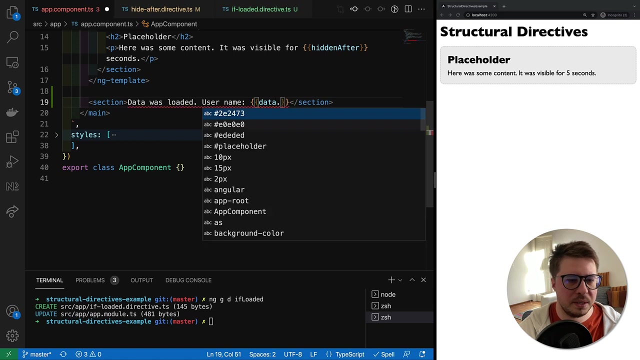 otherwise we should clear our view as easy as that, and now we have to apply the this directive in inside our app component. so somewhere here i will create a new section with username and there will be some data name right and we are going to apply if loaded and 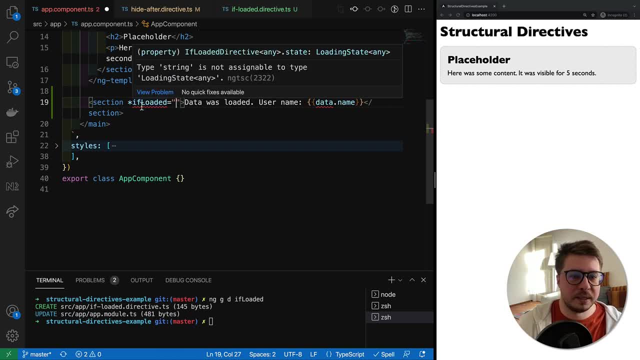 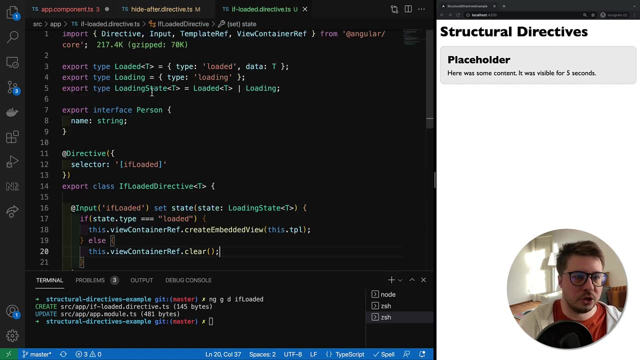 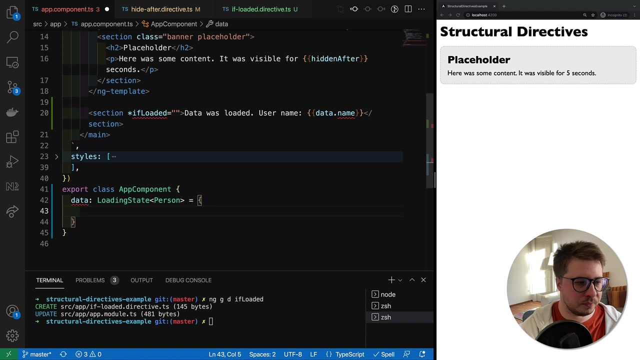 this: if loaded directive takes some loading state, so let's create it. uh, here it's a loading state, it is generic, and let's say that we are loading person, yeah, the person which comes, uh, from here. so this interface, by default it's going to be type loading, right, and then maybe 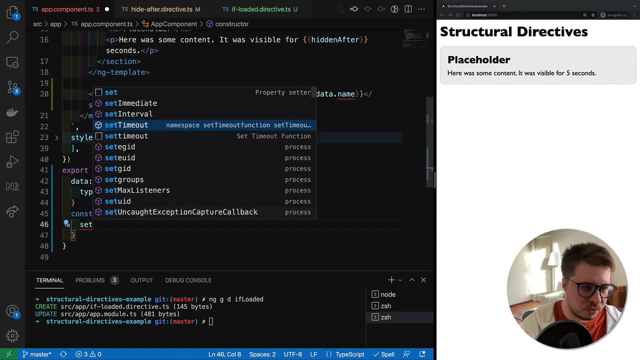 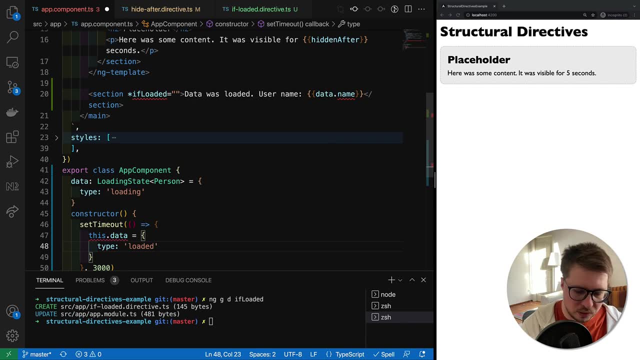 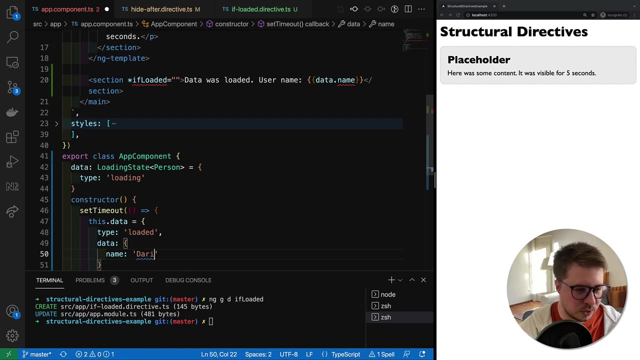 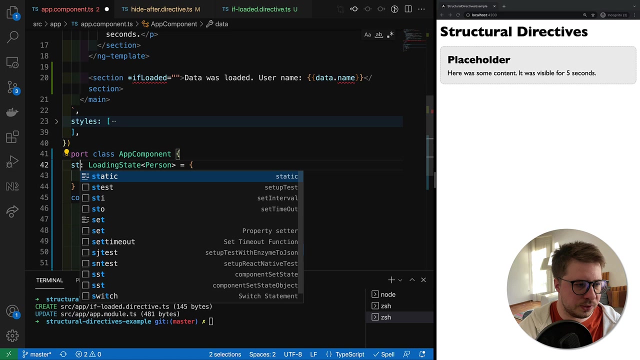 somewhere here we set timeout, we assign to the data some fake data and we say that type is going to be loaded and data is some user. let's use the name of my sweet wife and, ah, we have to. let's rename it to maybe state better state, and here should be state. 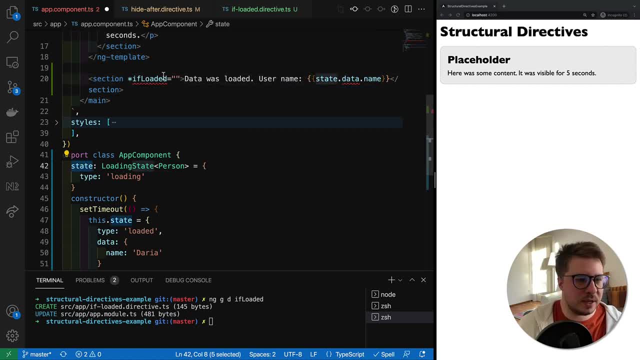 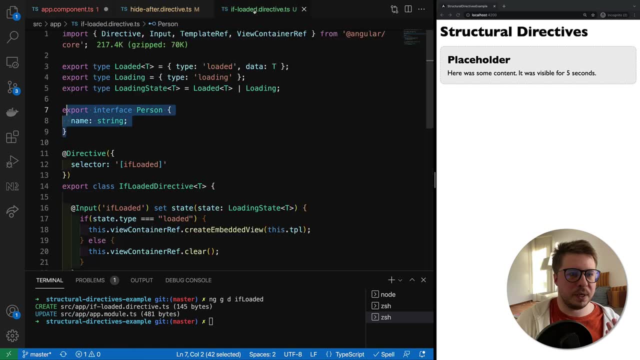 date name, all right, and we have to provide this state as the argument for our if loaded. so pretty simple. we have a state which might be: uh, either object which has loaded, type loaded and some data, or it can be the object which has only type and equal to loading, yeah, and. 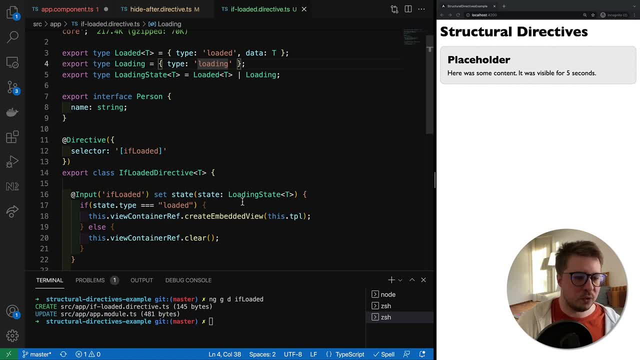 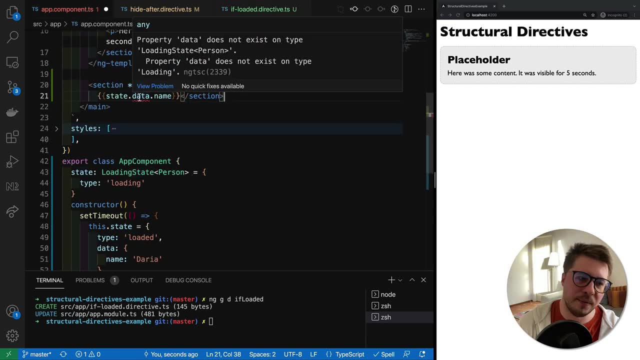 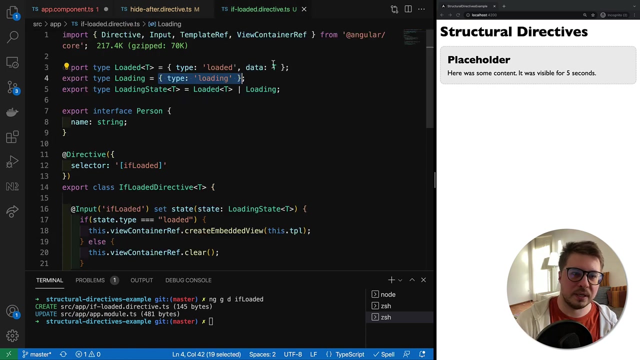 uh, the argument for if loaded input could be either either this or that. so we're using union type right here and you can see right now that we have an error which says that property data doesn't exist on type loading, and indeed our state might be either loaded which has, uh, this data type. 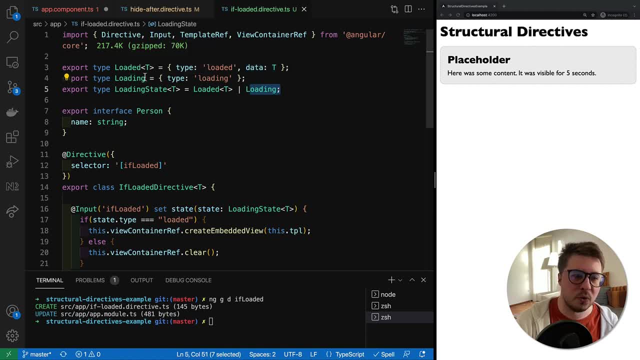 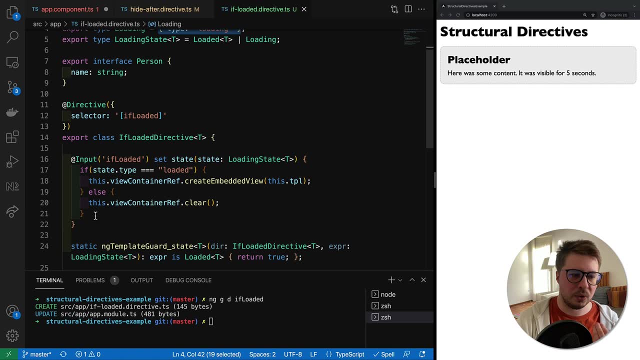 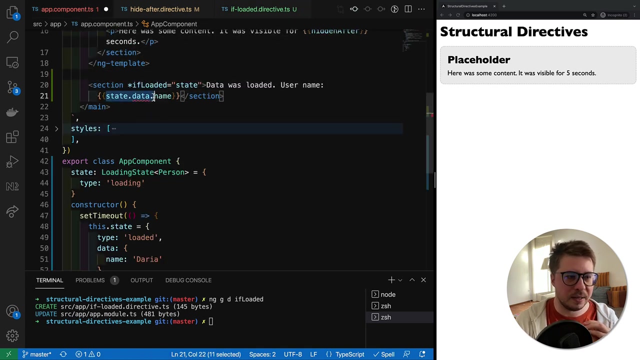 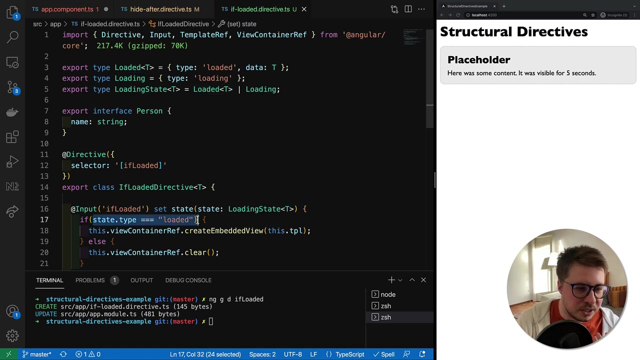 or it might be type loading, which doesn't have this uh data property. but we know, according to our logic, which we defined here, that when we generate the template, the type of if loaded means the type of this part will be always loaded. yeah, we check it here and we create the view only if it's loaded. 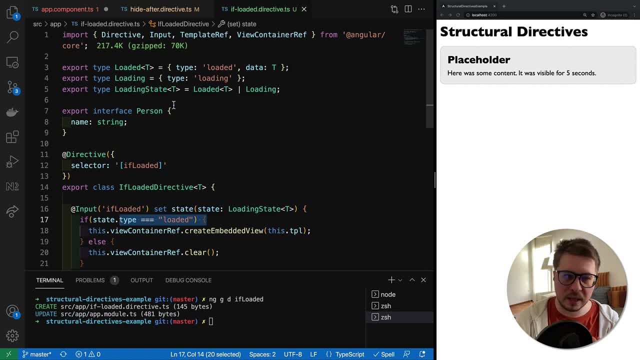 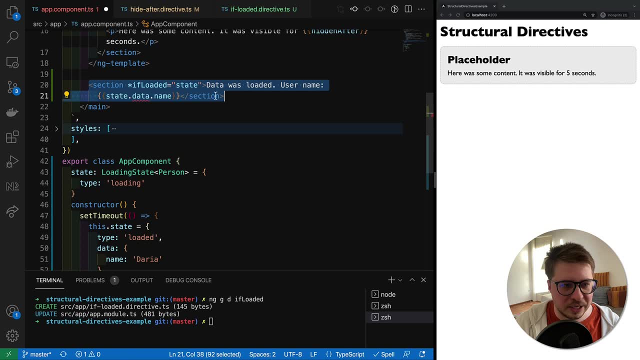 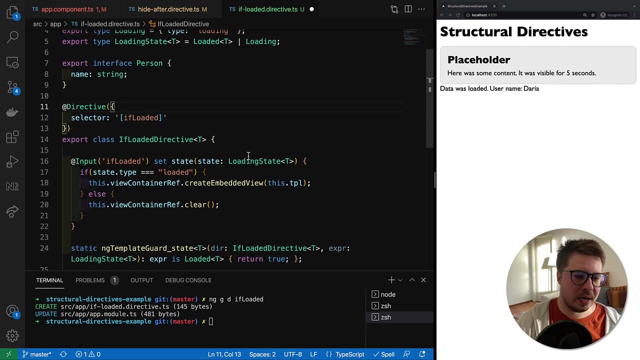 so we can give a hint to angular compiler that if we use the orientation visto the moderator, our state inside the this section where this if loaded directive is applied, then consider state of type loaded. and in order to achieve this we have to use another static method which has the following naming convention: it starts: 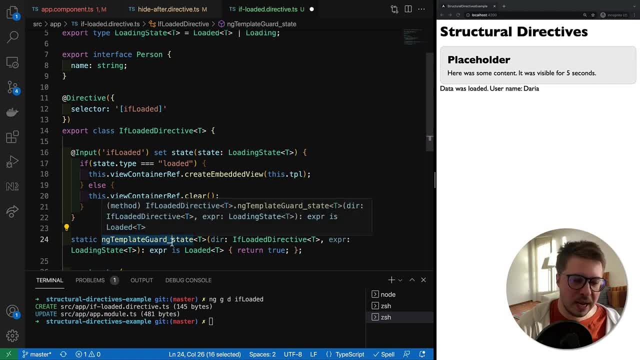 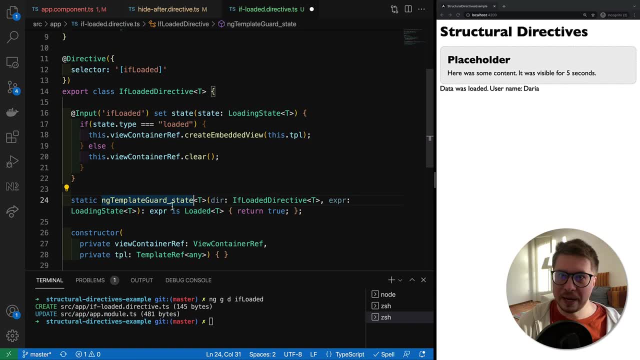 with ng template, guard and underscore and then there should be the name of the input, and you may wondering why it doesn't work. so we have this static method. the problem is that there is a small mistake in official documentation page right here. the problem is that if you use construction like this, the 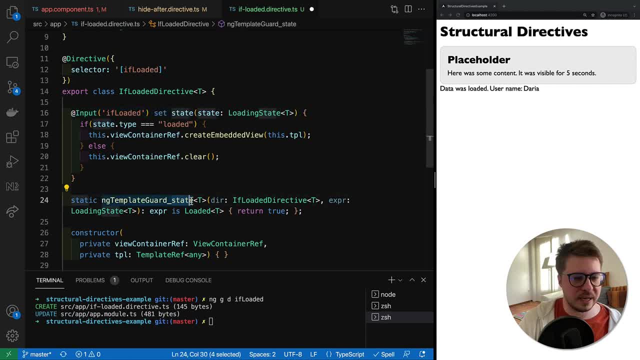 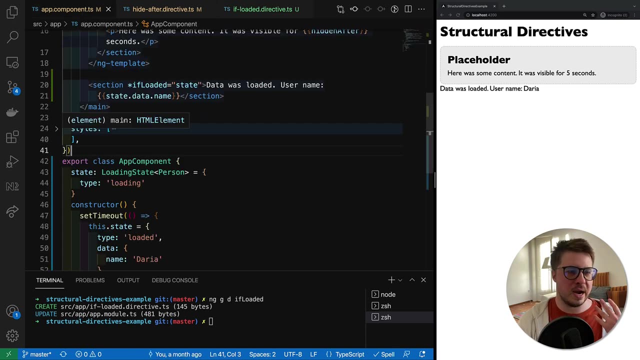 second problem is, for example, that we have to build this of like this: so this part of this static method name should match not the setter name, but rather the input name. so you have to replace it like that and now, if we save it, you can see that our error from the template. 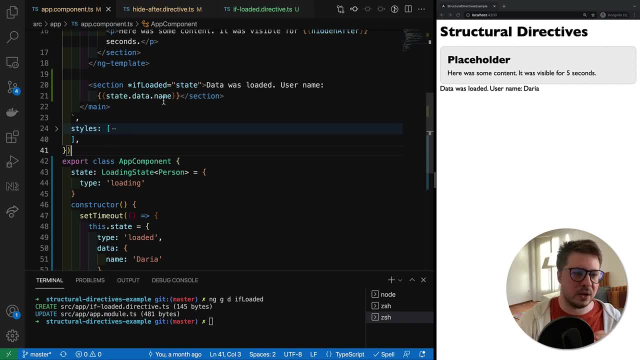 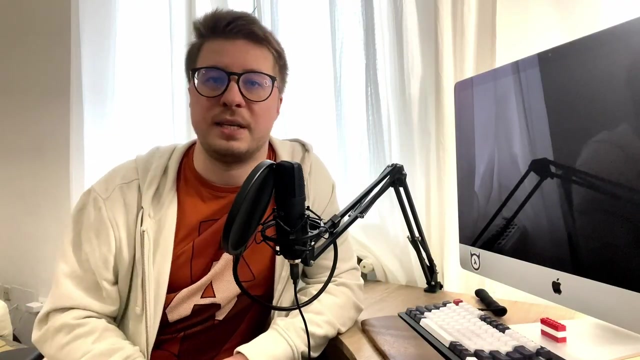 is gone and angular compiler treat the state as a loaded always because we gave a hint to it that inside the template, please consider that the type of state will be always, uh, kind of loaded right. all right, guys, that was it. thanks for watching until the end. i really hope that you learned. 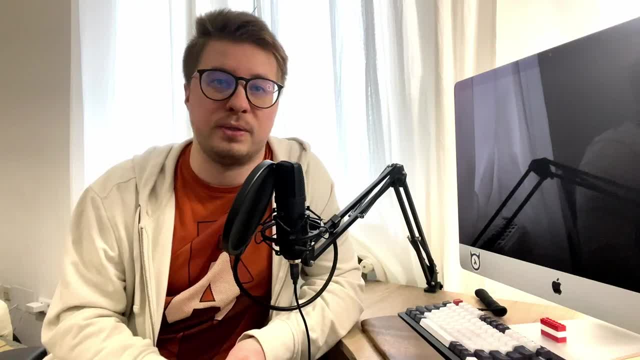 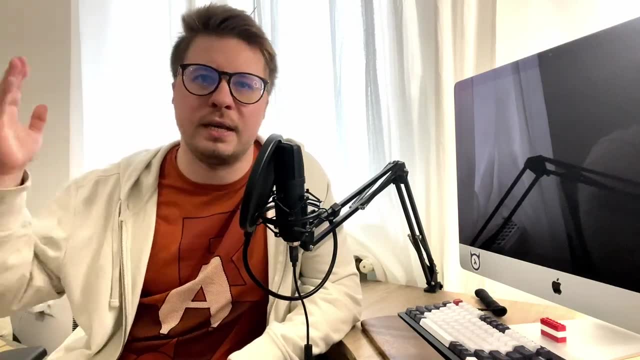 something new today. also, don't forget to leave your thoughts about the video in the comment section. and if everything, what i'm doing, my videos, everything if it makes sense to you and if you learn something new, please let me know in the comment section and i'll see you in the next video.